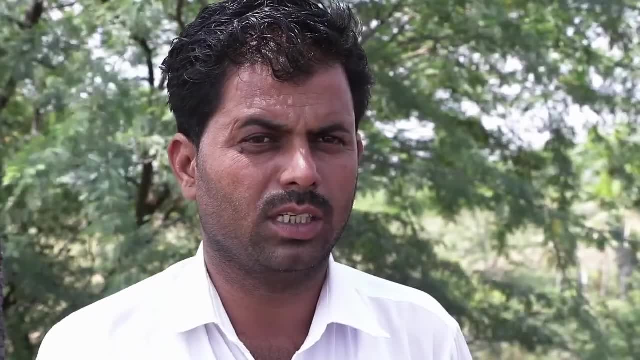 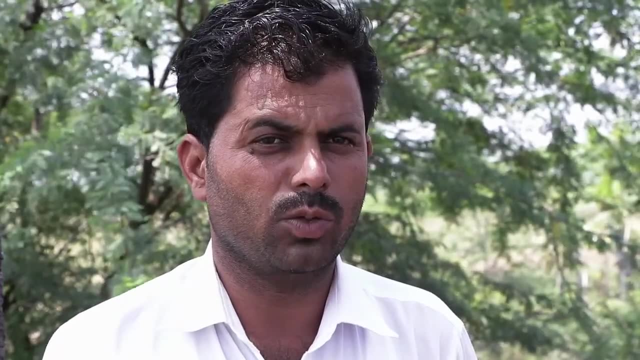 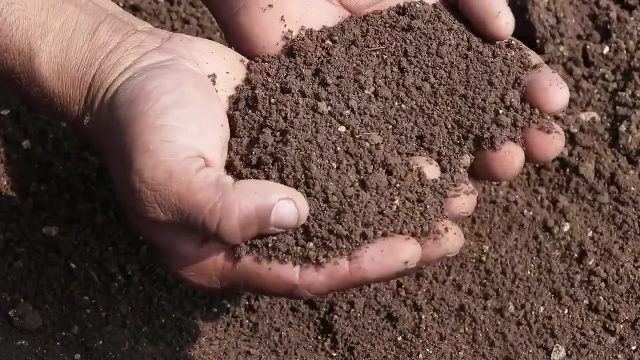 things in the soil. This makes the soil hard. Every year I had to use more chemical fertilizer and pesticides. We found it difficult to keep up with the demand of the soil to get more yields or even the same yield. Healthy plants require healthy soil. A healthy soil contains many kinds. 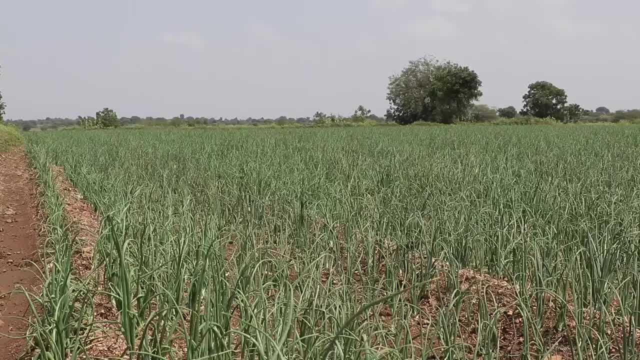 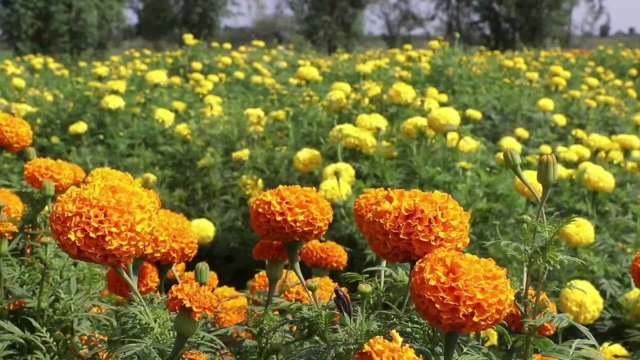 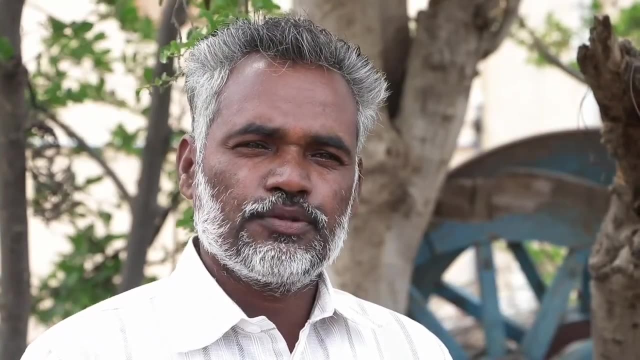 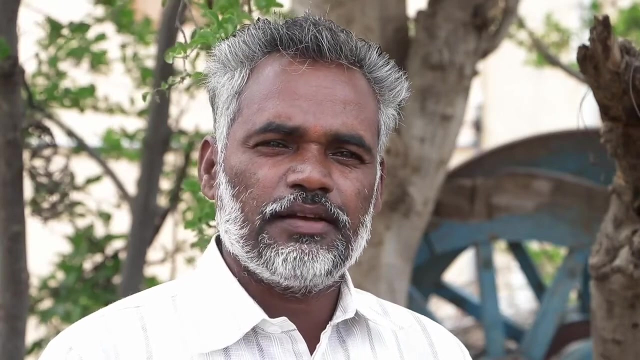 of living organisms, including good microbes that nourish plants. These good microbes enrich the soil and protect plants from diseases. But chemicals kill these good microbes. Good microbes make the soil loose and help to make the soil richer and more fertile. Plants grow better when I increase good microbes in the soil. 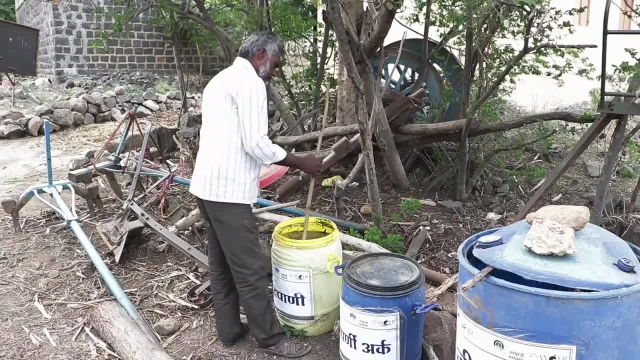 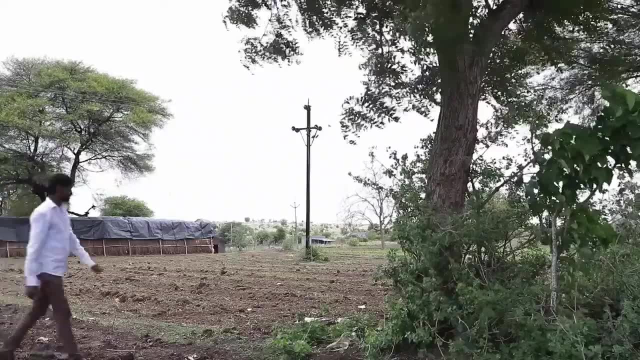 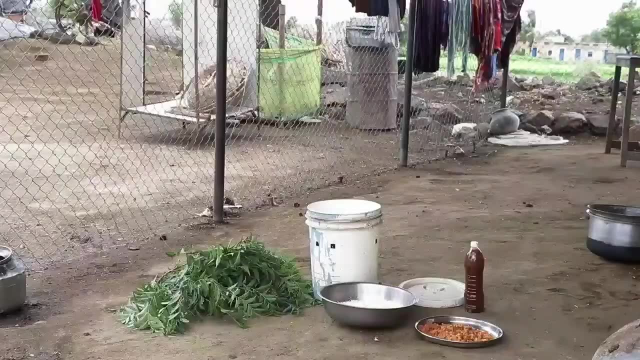 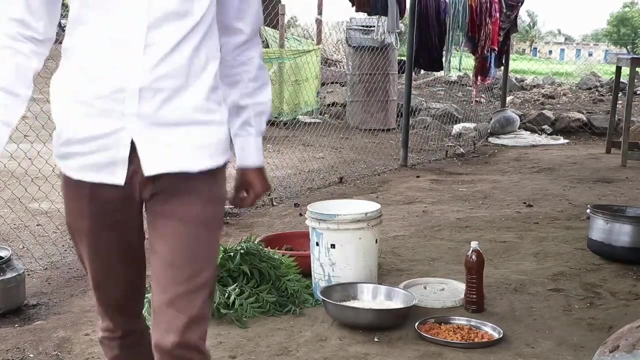 Farmers in India prepare various kinds of organic solutions to help beneficial microbes to grow in the soil. They make organic solutions from locally available ingredients at low cost to enrich the soil and increase yield. In this video, we will learn about a solution that boosts the crop's growth and, at the same time, protect the crop from pests and diseases. 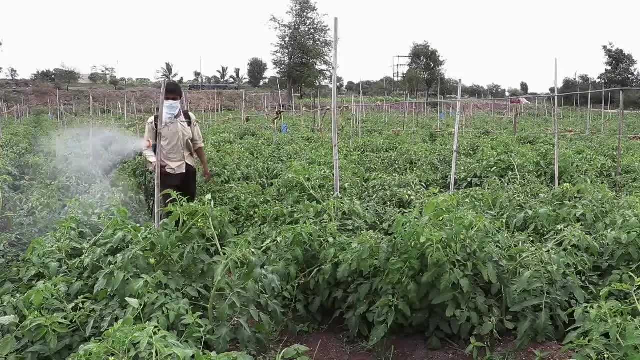 Over time. applying chemical fertilizers and pesticides can help the soil to grow better. This can be done with the help of chemical fertilizers and pesticides. This can be done by applying chemical fertilizers and pesticides. by applying chemical fertilizers and pesticides, Thermal fertilizers and pesticides kill the good microbes in the soil and can make the 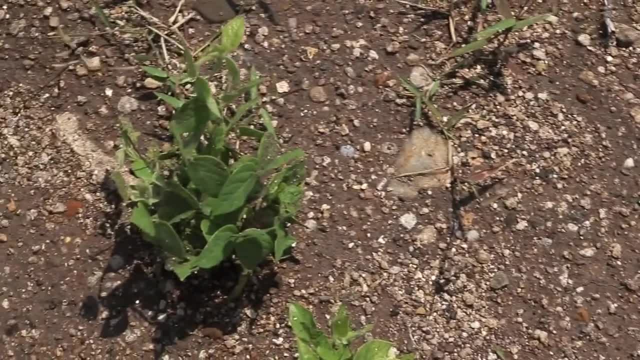 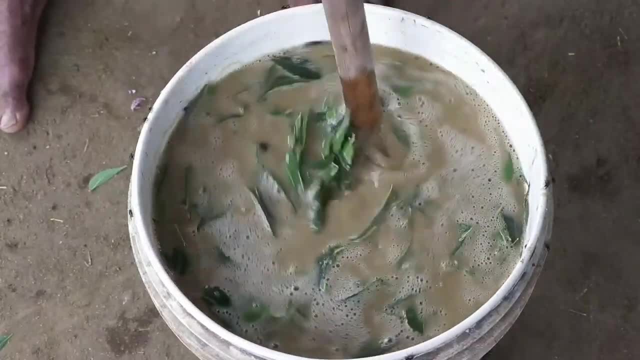 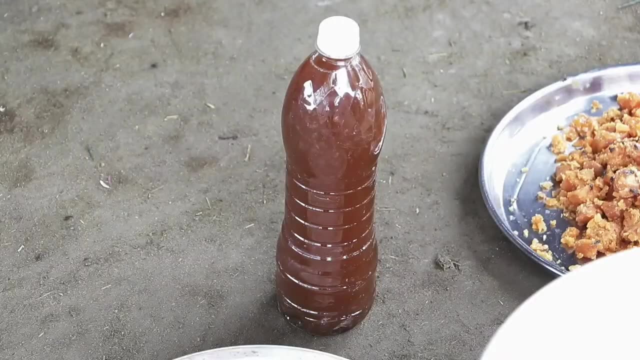 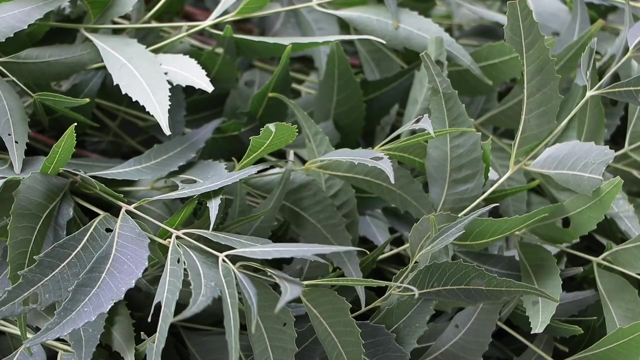 soil hard, so plants can no longer grow healthy. We can prepare an organic solution which will enrich the soil and help the crop grow better. Mix fresh cow dung, cow urine, water, proteins and some raw sugar. You can add bitter leaves if you want to control pests at the same time. 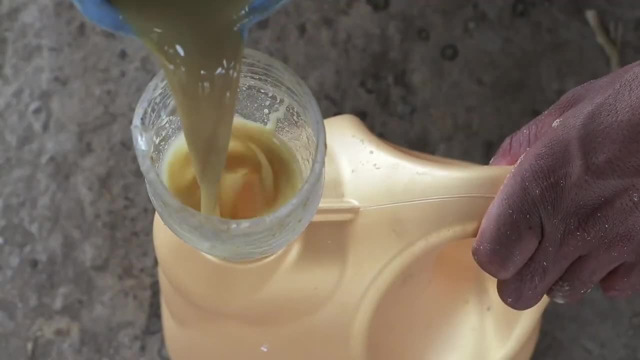 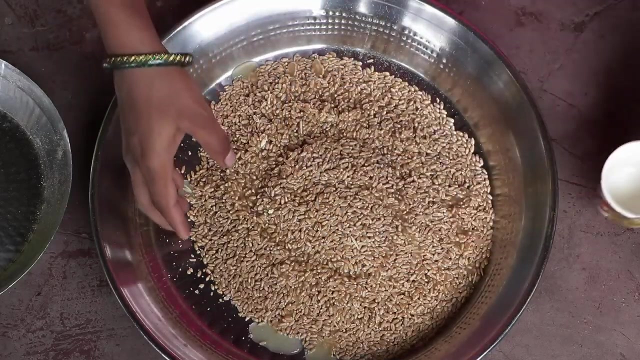 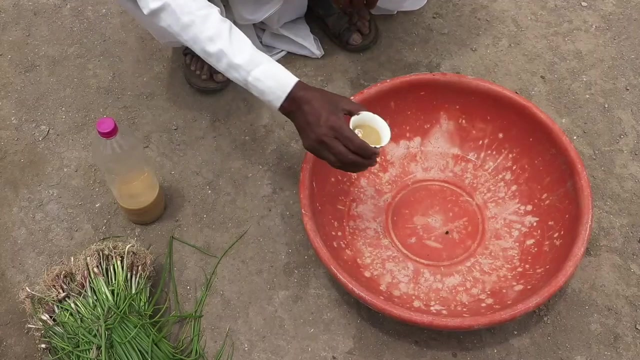 After 10 days, filter the mix and store it in an airtight container. The filtered mix can be used for seed treatment. Treated seeds will germinate better and resist pests and diseases. You can also use the filtered mix to encourage roots to grow.